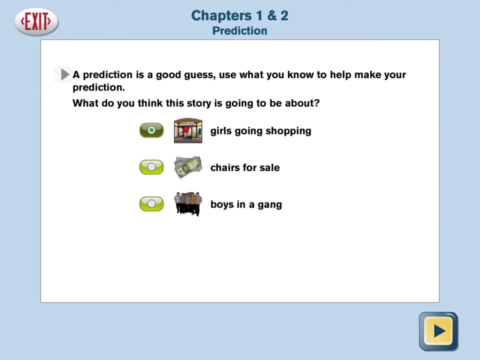 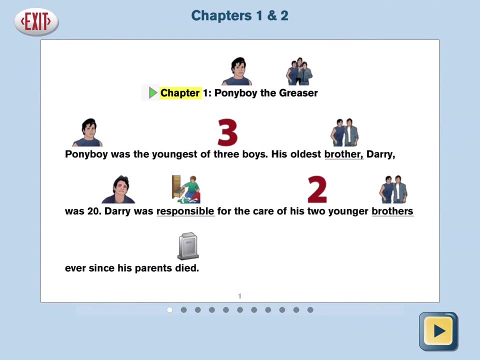 Tap to make a prediction. The first test question will revisit the answer chosen here. Read Chapter 1.. Ponyboy the Greaser Ponyboy was the youngest of three boys. To pause the narration, tap the screen To read the page again. 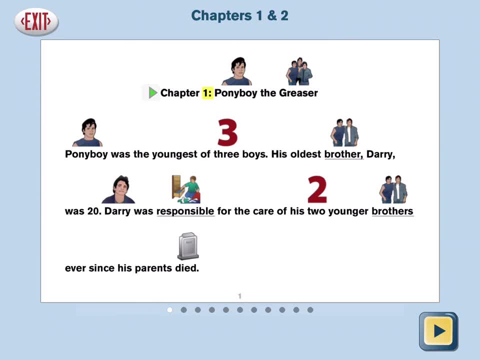 tap the play icon at the beginning of the line, Chapter 1. Ponyboy the Greaser Or double-tap any word to resume reading. at that location, Derry was responsible for the care of his two younger brothers. Single-tap a word to hear it spoken. 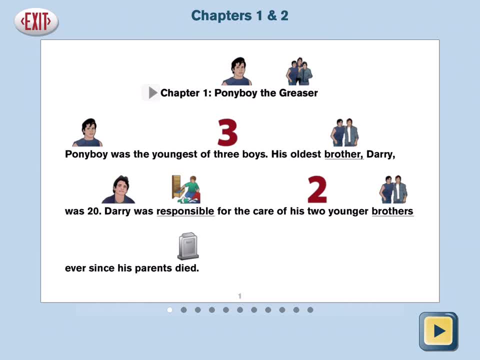 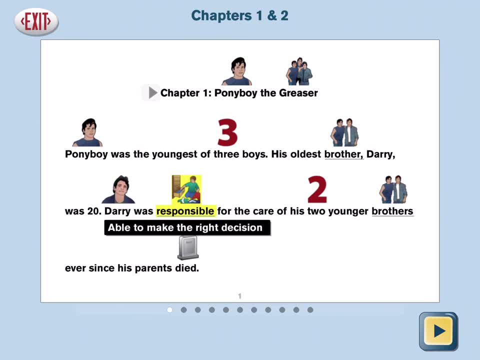 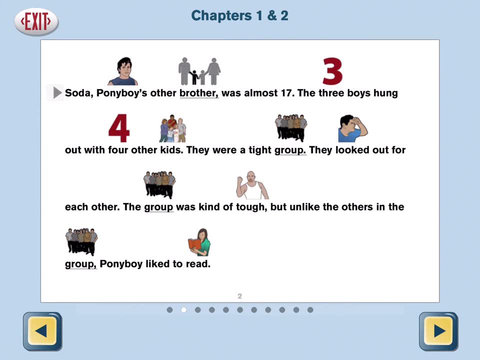 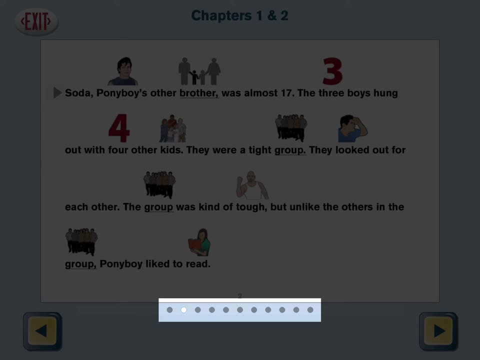 Tap the underlined word to see and hear it spoken. Able to make the right decision. Turn the pages forward or back by tapping the left or right directional arrows at the bottom of the screen To jump ahead or back. multiple pages touch, pause slightly, then release on a page, dot. 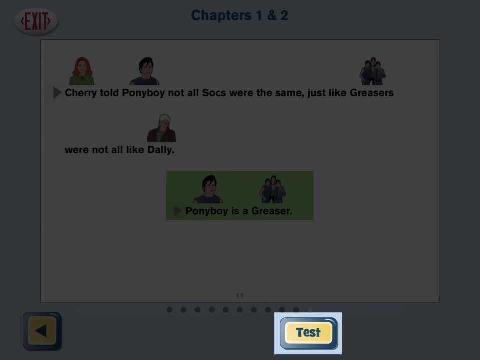 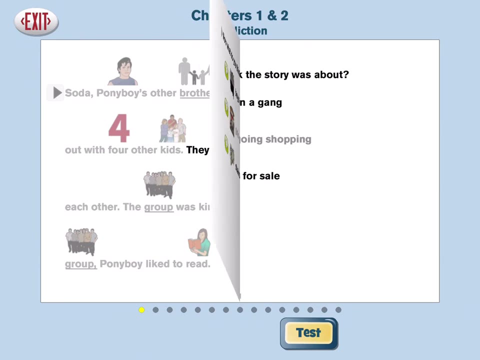 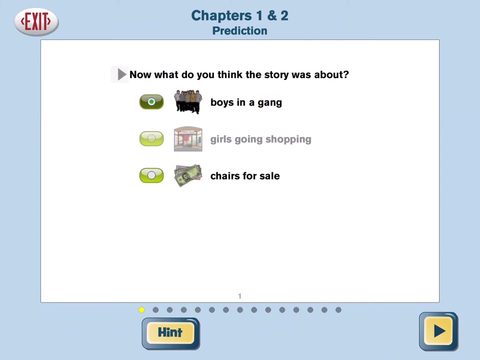 The last page of the read activity has a test button. Tap to begin the questions. Tap the Hint button to hear a hint. The Hint button takes the student back to the page containing the answer. Selecting an incorrect answer takes the student back to the same page and highlights the appropriate sentence. 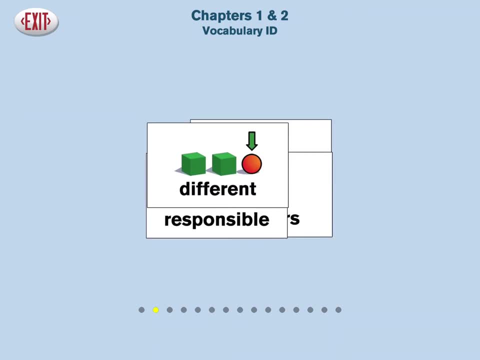 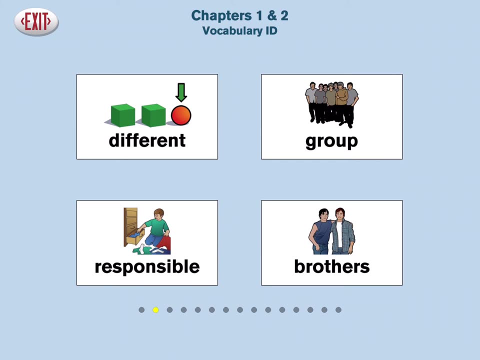 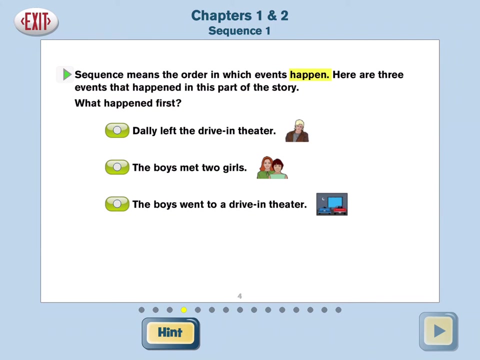 Testing Vocabulary: Identification and Vocabulary Meaning is next. All four words are quizzed for both identification and meaning. This is followed by sequencing questions. The sequencing questions are followed by nine multiple-choice comprehension questions, including main character, setting, problem and solution. 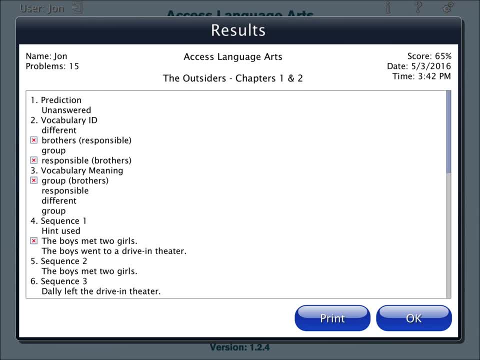 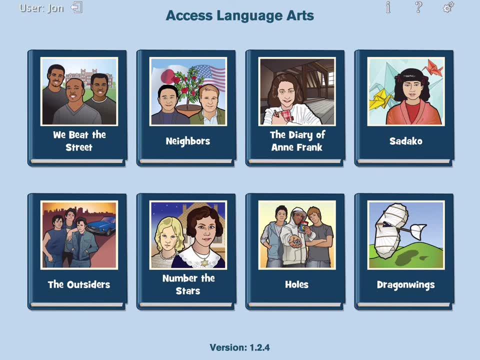 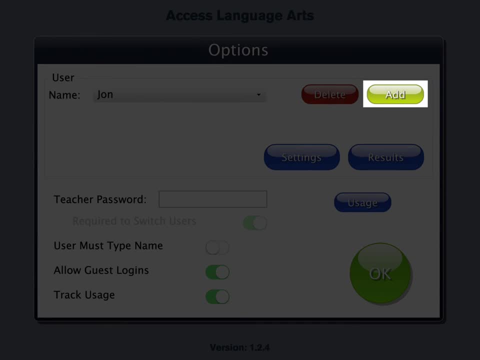 Results are shown after completing the questions. To add a student account, adjust user settings or view resources, tap the gear icon. To add a student account, tap the Add button, type the student's name and tap Next. The teacher password allows you to create an optional password that needs to be typed to open options. 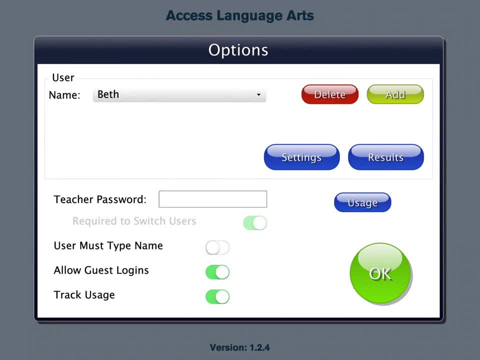 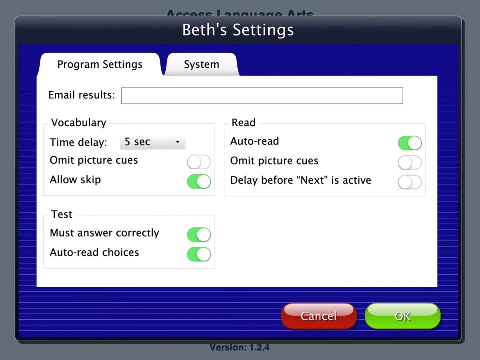 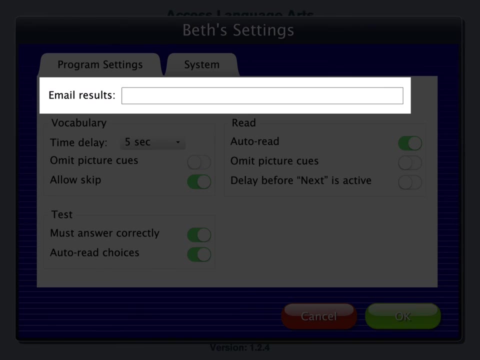 To adjust a user's settings, select the student's name from the drop-down menu and tap Settings. The app has two tabs and settings: Program Settings and System Email Results. Details of the student's test results are shown at the end of each test. 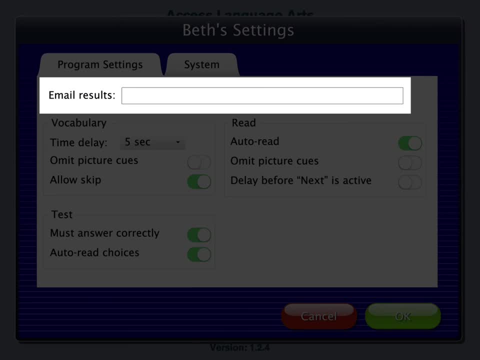 When an email address is entered in this field, an email will be generated at the end of each test with the detailed results. Vocabulary Time Delay: Set the amount of time to transpire before the verbal prompt is repeated. Omit Picture Queues. The default is Off, which means words are presented with Picture Queues. 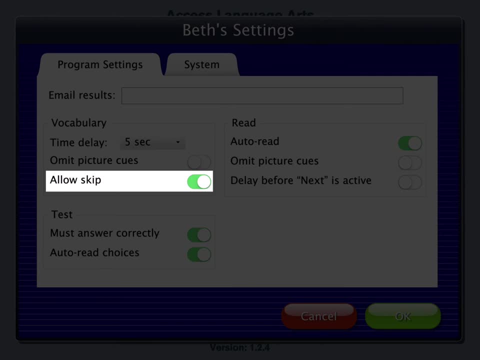 Turn it On to remove Picture Queues. Allow Skip. The default is On. This allows students to advance past Zero Time Delay or Vocabulary ID by tapping the forward arrow Under Test. the default for Must Answer Correctly is On. This requires the student to select the correct answer before moving on to the next test question. 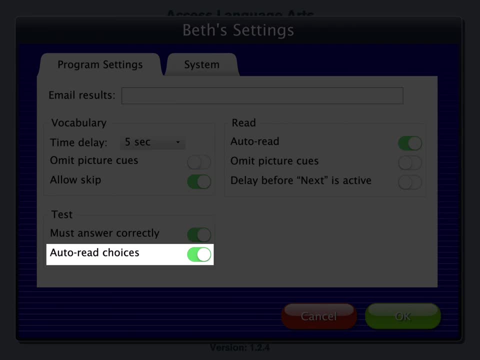 Auto Read Choices: The default is On. This reads the answer choices right after reading the question. Auto Read Default is On. Narration will begin automatically upon starting a new page. Omit Picture Queues. The default is Off. If turned On, symbols are removed from the Preview and Read activities. 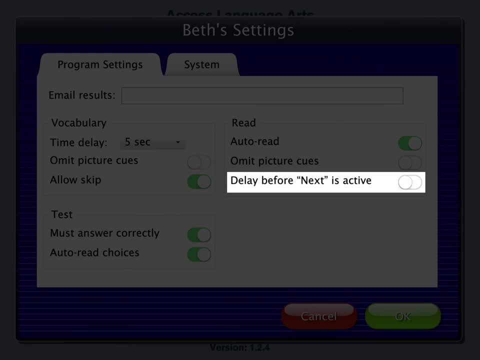 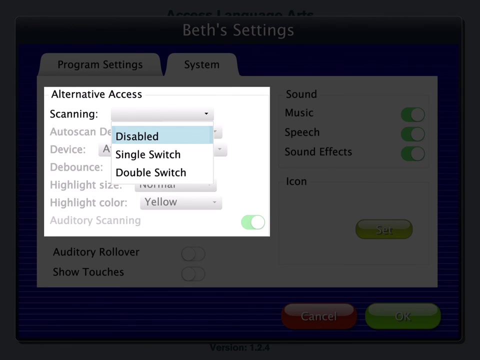 Delay Before Next is Active. The default is Off. If turned On, there will be a slight delay before the student can manually advance the page by tapping the forward arrow. Built-in Scanning provides program access with switches To use Scanning. select one or two switches.